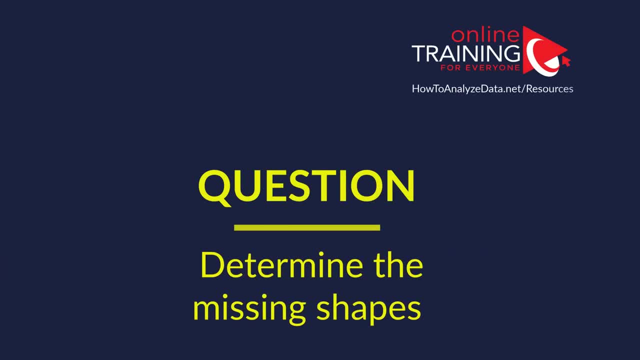 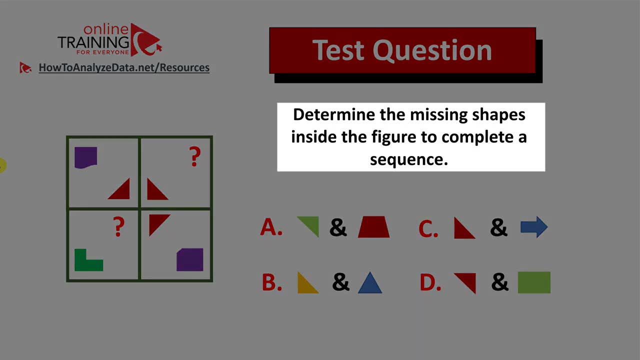 Let's look at the interesting question which tests your pattern recognition skills: Determine the missing shapes inside the figure. to complete the sequence, In your presented with 2x2 figure, it has two missing shapes and you have four possible choices: A, B, C and D. Do you see the answer? Now might be a good time to pause this video and give yourself. 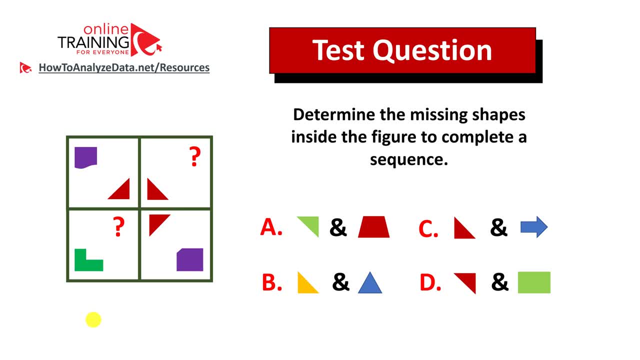 10 to 20 seconds to see if you can come up with the solution on your own. Did you figure out the solution? Let's continue to see how we can solve this challenge together. As usual, to solve these types of problems on the test, you need to look for patterns, And there are. 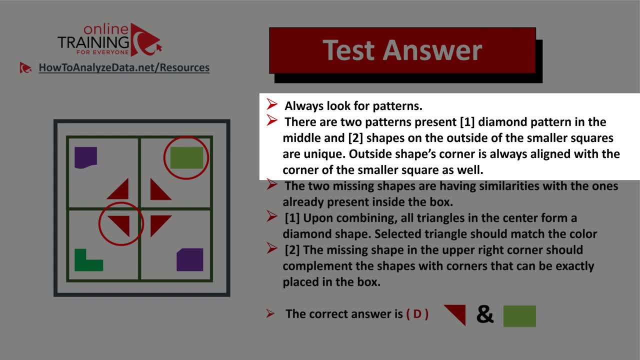 two patterns here presented. Number one is the diamond pattern in the middle And number two is the pattern of shapes on the outside of the smaller squares, which are unique Outside shapes. corners are always aligned with the corner of the smaller square as well. The two missing shapes. 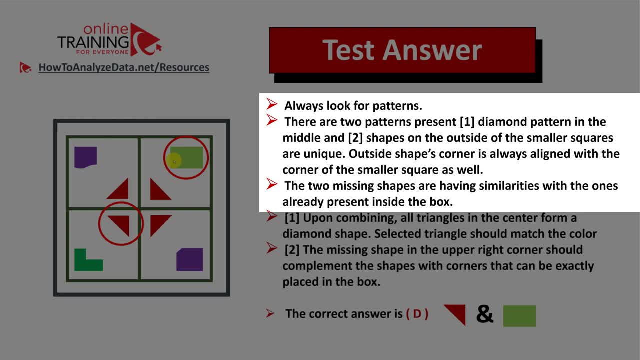 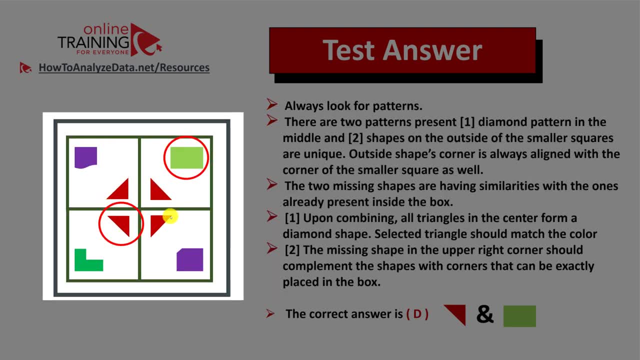 also have similarities with other shapes present in the box. Upon combining, all triangles in the center form a diamond shape. Let's look at each one of these two patterns in more details. You should look for the triangle which matches the color And, upon combining it should build a. 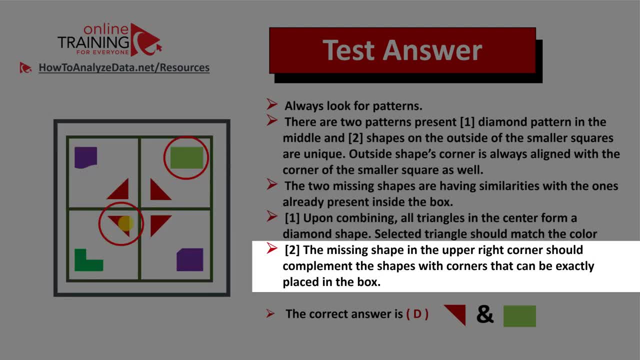 diamond. For pattern two, the missing shape in the upper right corner should complement the shapes with the corner of the smaller square And you should look for the triangle which matches the color And you should look for the triangle which matches the color of the smaller squares. 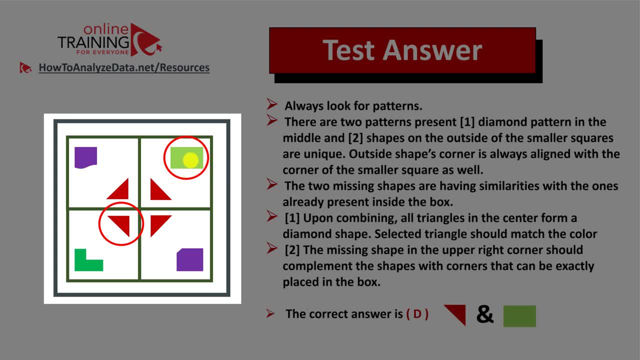 In this case, we selected green rectangle. You also notice that there is a pattern of green color on the opposite side of the squares, same as the purple colors on the opposite sides of other squares. So the correct answer here is choice D. Hopefully you've nailed this question. 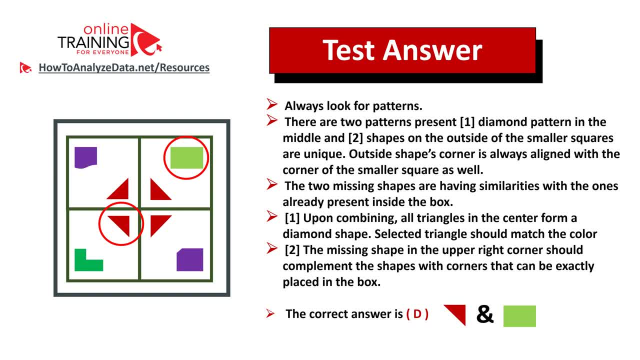 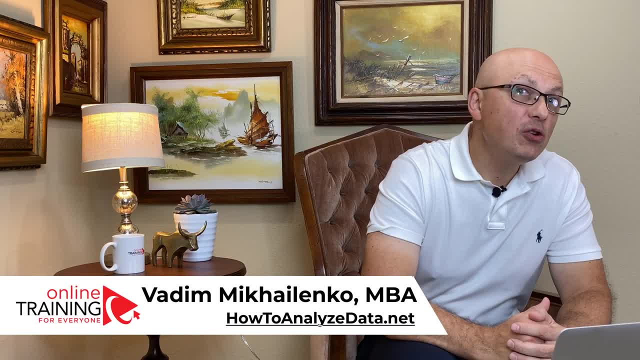 and now know how to answer similar questions in the test. Thanks for watching. I encourage you to check out our daily question challenge in the community section of this channel. I also recommend that you check out the video description below. If you find it useful, please like and subscribe. 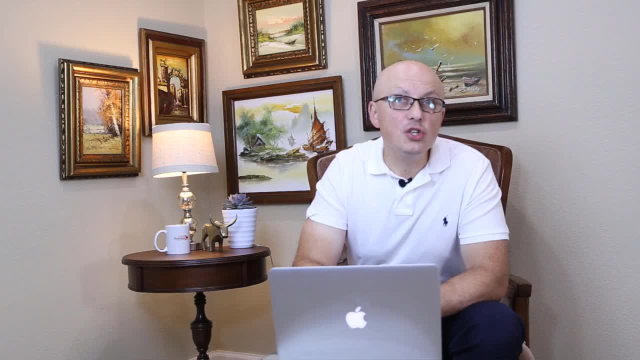 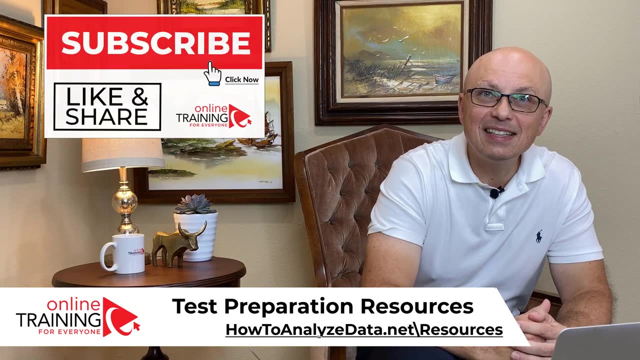 and check the downloads in the description section of this video. Please also check out the resources page on our website, howtoanalyzedatanet slash resources. If you like the content, please give this video a big thumbs up. This tells us that you need more content like this. I would encourage you.